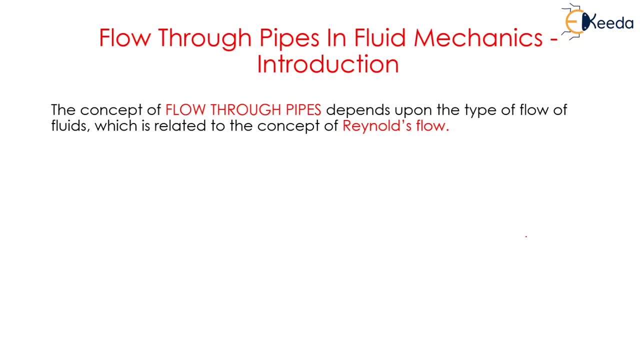 So what is Reynolds flow? A scientist named as Reynolds gave a number which is known as Reynolds number And based on that we have classified some flows. So the ratio of inertia flow to the viscous flow is termed as Reynolds number, And if the Reynolds number is less than 2000, then the flow is said to be laminar flow. 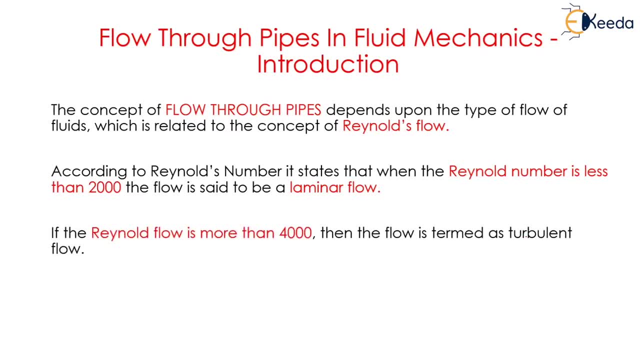 So when the Reynolds number is greater than 4000, then I can say the flow is said to be a turbulent flow, And if the Reynolds number is in the range of 2000 to 4000, the flow is termed as transition flow. So we have learned about three different flows, namely laminar flow, 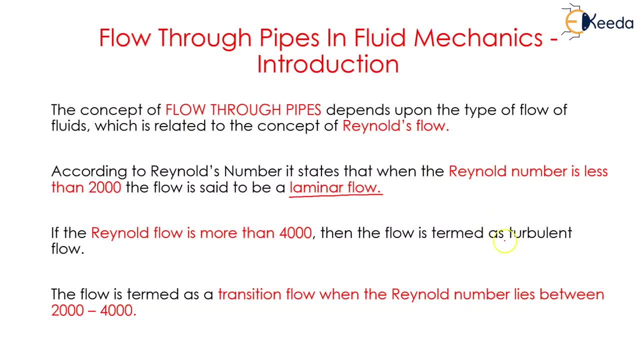 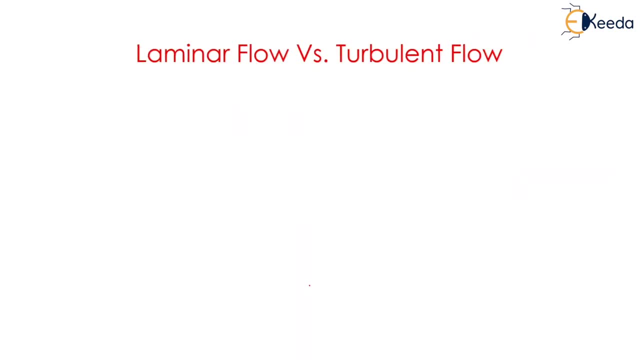 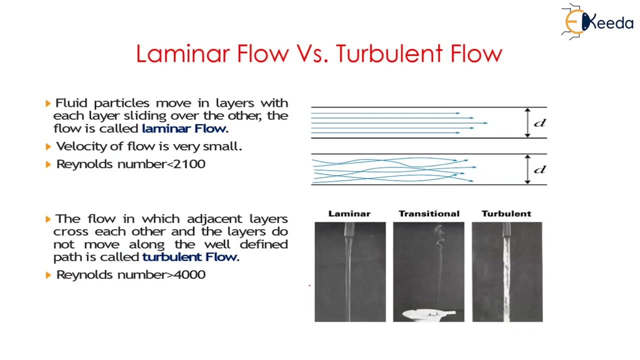 The next one is turbulent flow And the last one is transition flow. So, based on this, we have to study what is flow through pipes: Laminar and turbulent flow. So just now we studied: when the Reynolds number is less than 2000, the flow is said to be laminar flow. 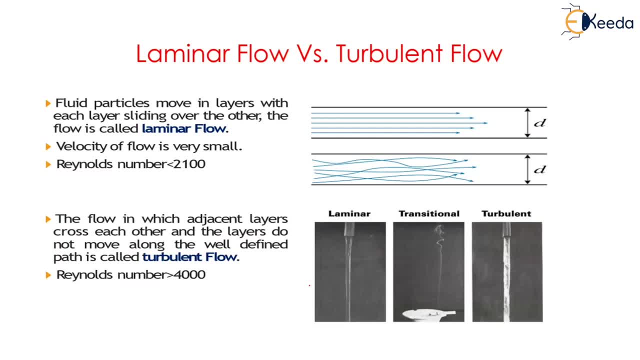 And if it is greater than 4000 the flow is said to be a turbulent flow. We have just classified the flows but we need to study how the flow functions. So in laminar flow I can say the first diagram over here is for laminar flow and this second diagram shows the flow as turbulent flow. 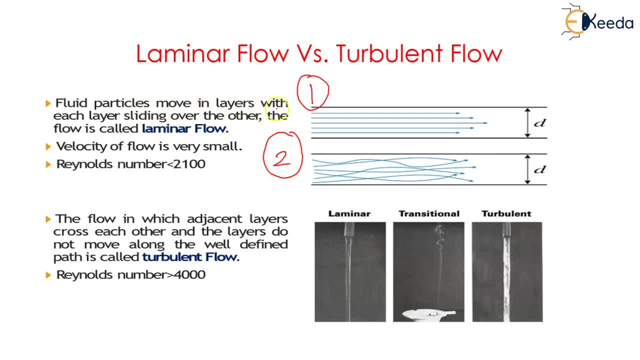 What it means. The fluid particles move in layers, with each layer sliding over the other. The flow is said to be laminar flow. In this I can observe the fluid particles flowing over each other- do not cross each other- But while I can see in the second diagram or second figure that the particles of flow cross each other, 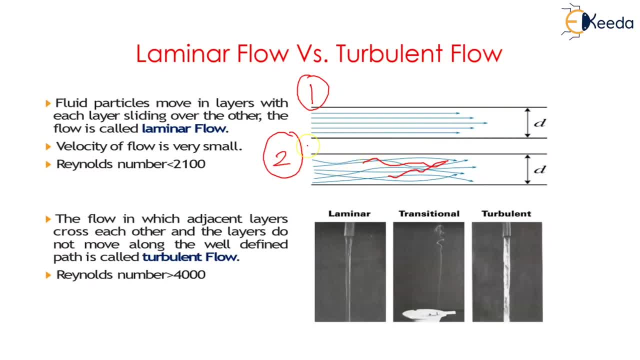 So this kind of flow is termed as turbulent flow, While the layers sliding over each other and not crossing each other is termed as laminar flow. So the velocity of the flow for laminar flow is very small, While that for turbulent flow is large. 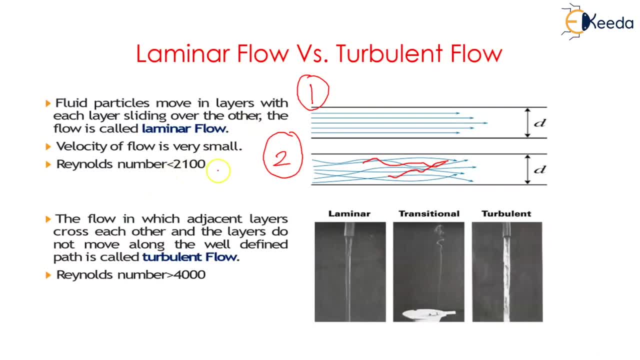 Reynolds number is less than 2000 or I can say 2100. And over here the Reynolds number is greater than 4000 for turbulent flow. So in this next image I can see we have given three different flows. The first is laminar flow. 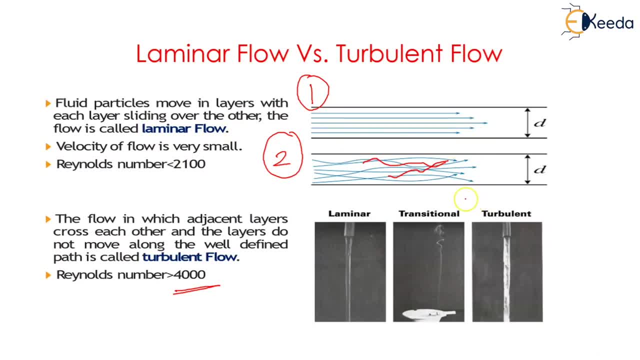 The second is transition flow And the third is turbulent flow. In this, I can say, the velocity of the liquid or flowing water is very less And the layers of the fluid do not cross each other. It is flowing in well defined manner, While when the velocity increases, that is, in the case of turbulent flow, 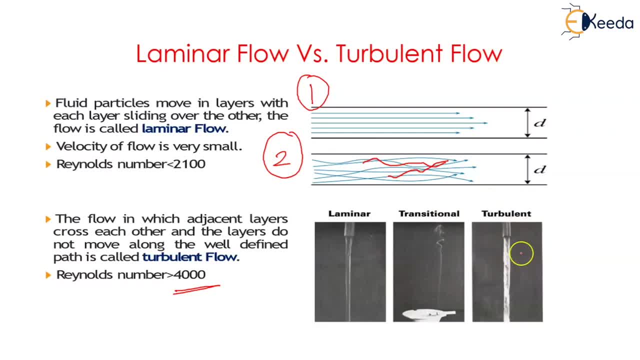 I can see some of the particles of fluid do cross each other And in this transition flow in the bottom side, I can say the flow is in a well defined manner, While once it reaches a certain level the particles crosses each other, And hence I can say, when two flows are in, combined in a single flow. 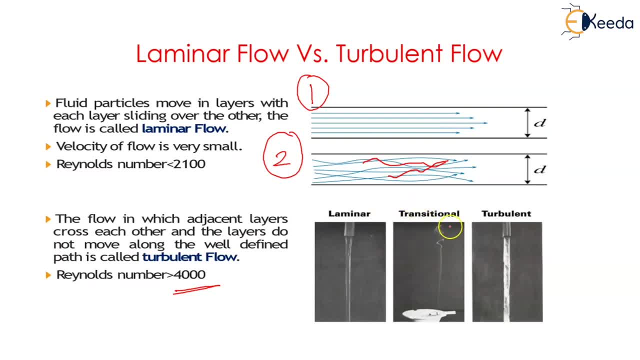 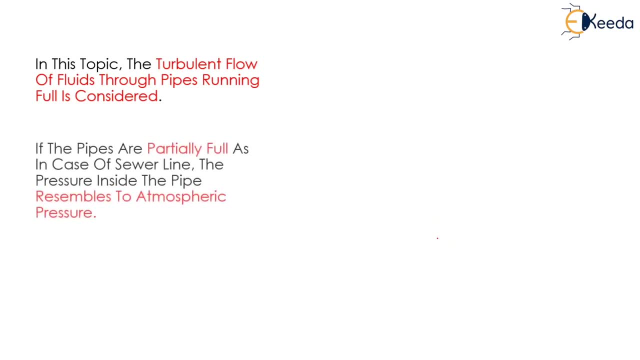 Then that kind of flow is known as transition flow. In this topic the turbulent flow of fluid through pipe running full is considered. If the pipes are partially full, as in case of sewer line, The pressure inside the pipe resembles to atmospheric pressure. We can see in this particular image: 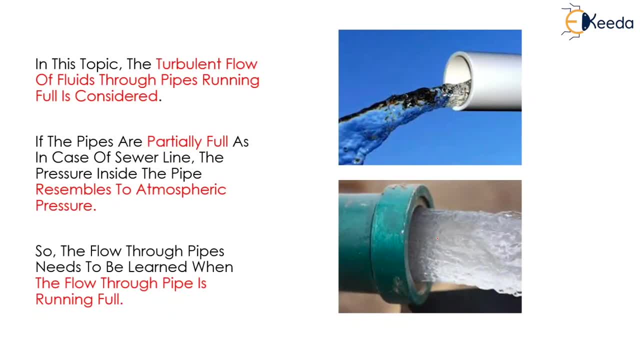 In the first image it is shown that the pipe is running half full, While in the second image it is shown that the pipe is running full. So the flow through pipe need to be learned when the flow through pipe is running full, As in case I can say in the first image. 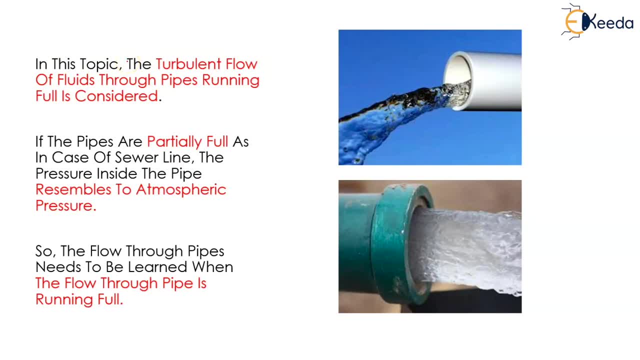 This is the case for sewer pipes And hence the pressure is atmospheric pressure. But in the second image I can see that the pipe is completely filled And hence the flow is under the pressure. So to study flow through pipes, we will focus mainly on the second condition.